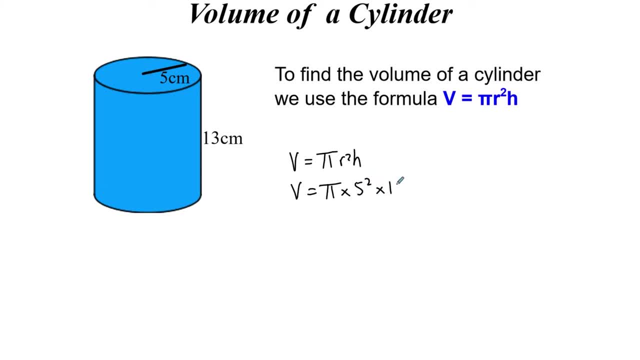 so that's 5 squared, in this case, times the height, which is 13.. Remember, sometimes, instead of giving you the radius, it might give you the diameter. so watch out for that. Type it into your calculator using the pi button, if you've got one. 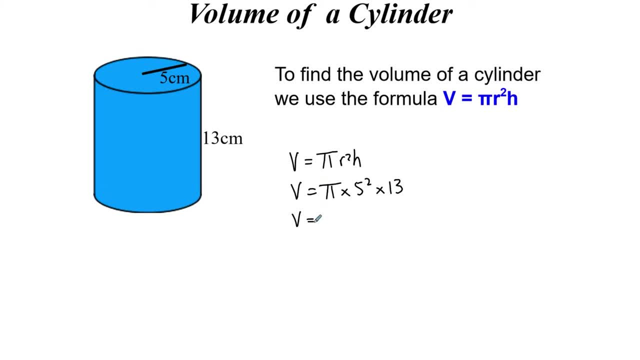 to get a nice, accurate answer, And it should give you 1021 point, and we'll just do it to two decimal places: 02 cm. cubed or cubic centimetres. Okay, so, very similar work into what we had for the volume of a cuboid or a cube. 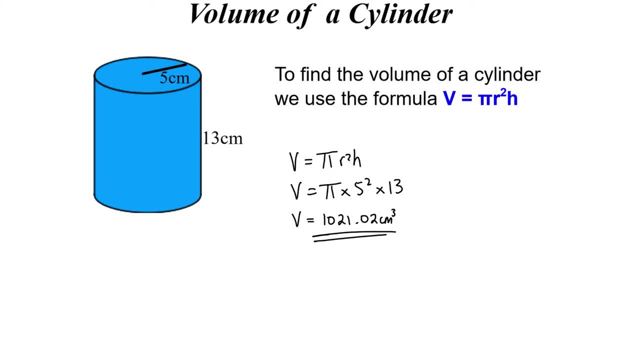 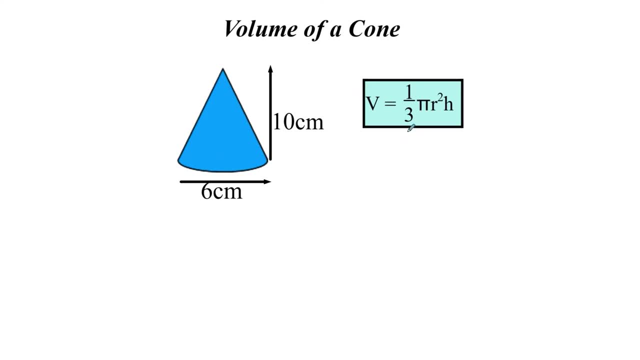 but obviously a different formula. Okay, let's have a look at the next page. So, volume of a cone. A cone actually looks a lot more complicated, but it's not too bad. It's basically just the volume of a cylinder, but it's a third of the size. 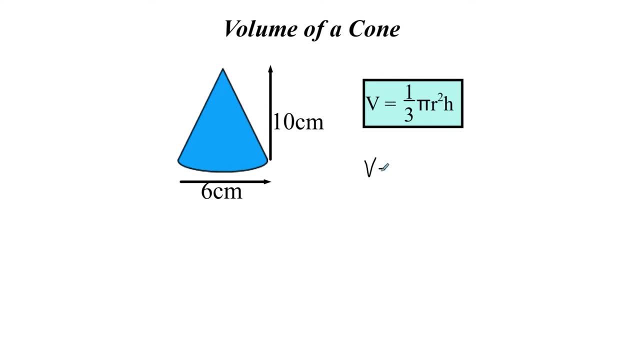 So it's a third pi r squared h. So write a formula down first: v equals a third pi r squared h. That's a third times pi times the radius. Okay, And this is what we have to be careful, Remember, the bottom part is your circle. so when we're looking for the radius, 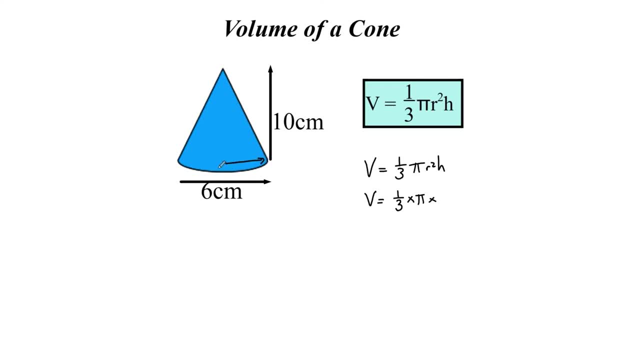 we're looking for the distance from the middle to the outside here, which would be three for a radius squared. don't forget, you're squared times the height, which is 10.. Okay, and again, we're just typing that into the calculator. 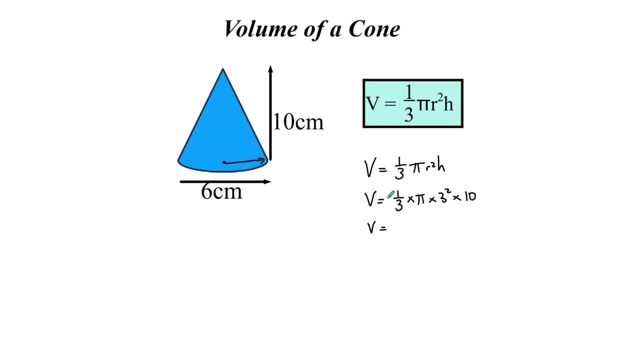 Now when you type that into the calculator, there's various different ways to do it. If you're not sure, just do it one divided by three, which is a third times the pi button, times three, squared, squared times 10.. 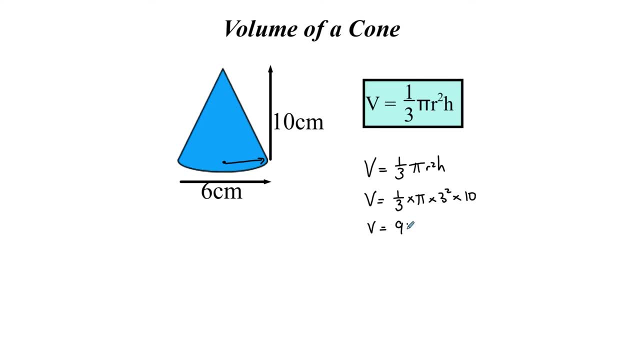 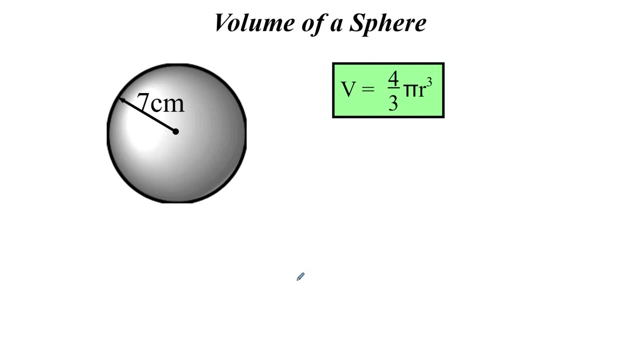 And that'll give you 94.25.. And again, we'll just stick to two decimal places. You could round differently and you might have to use significant figures depending on the question. See, I'm cubed, Okay. So last one we're going to look at before we move on to composite shapes is the volume of a sphere. 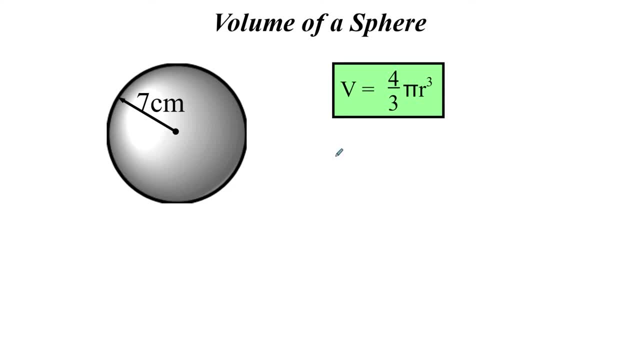 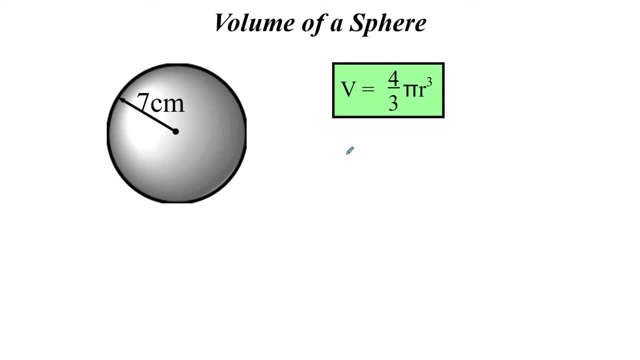 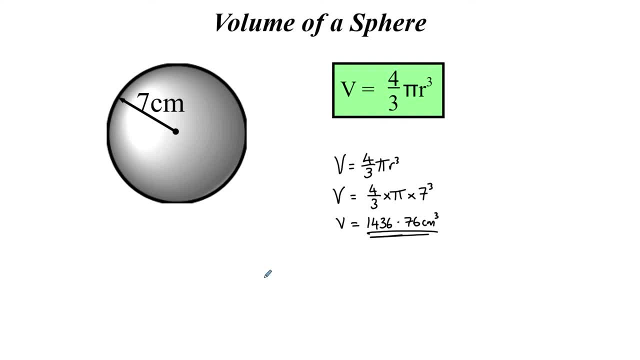 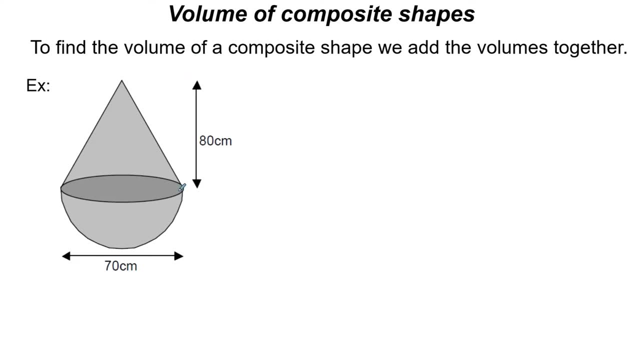 So now, and look a little bit at prisms and composite shapes. so, um, composite shapes are shapes that are just joined together. so we've got two basic shapes that we had, two or more basic shapes that we had have seen already, but they're joined together in some way. so here you can see, you've got a cone on. 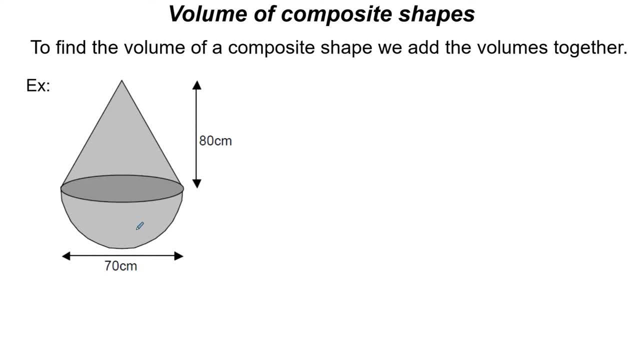 the top and a hemisphere or a half sphere on the bottom. so we're going to have two shapes we're going to have to calculate the volume of, so i'm going to label them one and two. so shape one- we're doing v- equals a third. remember each shape has its unique formula. so the cone is a third pi r. 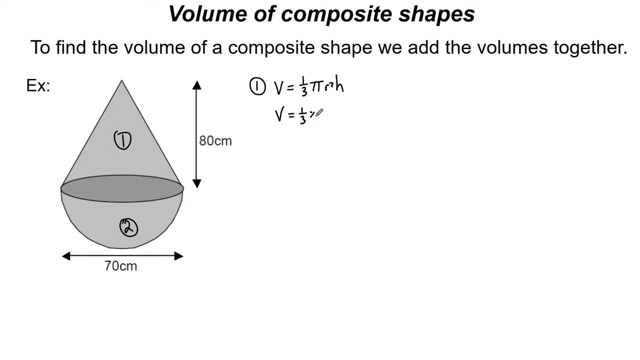 squared h. so it's the third times pi times. now the radius of this cone- this is what we're focusing on- is from here to here, okay, which wouldn't be 70, it would be 35. so times 35 squared times the height of the cone, which is 80.. okay, so it's 1 divided by 3 times pi times. 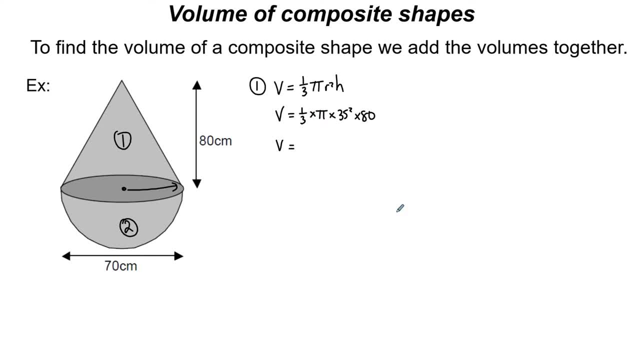 35 squared times 80, and that gives you 102 625 0.36 cubic centimeters. okay, so that's the first part. second part was the volume of the hemisphere. now it's up to you which way you want to do this. it is half a sphere, so we're still thinking of 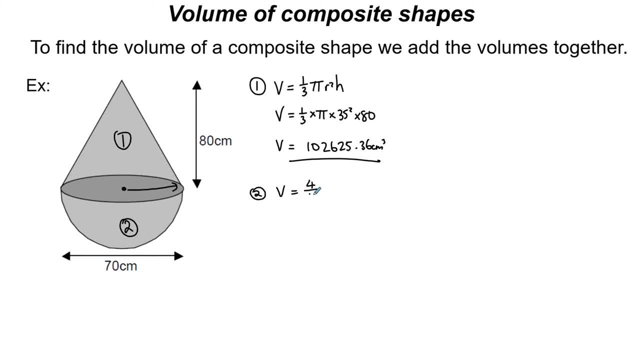 the, the volume of a sphere formula, which is four thirds pi r cubed, which we saw in the last page. but it's only a half sphere, so we've got to take half of that value. now i would just normally put the half in here, so you can either multiply it by half or divide by two. so i'm going to multiply. 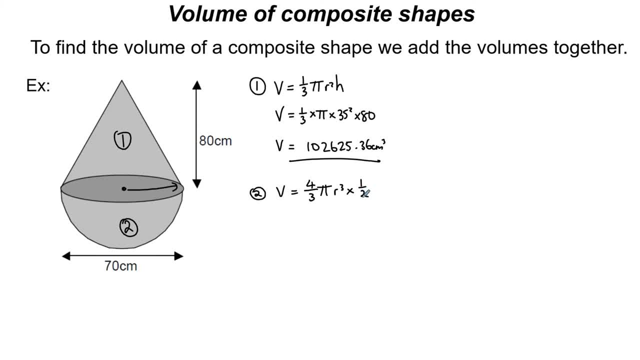 by a half at this stage, because it's only a half sphere, and that way we don't have to worry about it. for the rest, we just type it into the calculator and we're done so four thirds times pi times the radius of the sphere, or the hemisphere, which again is this distance here. so that would be 35 cubed. 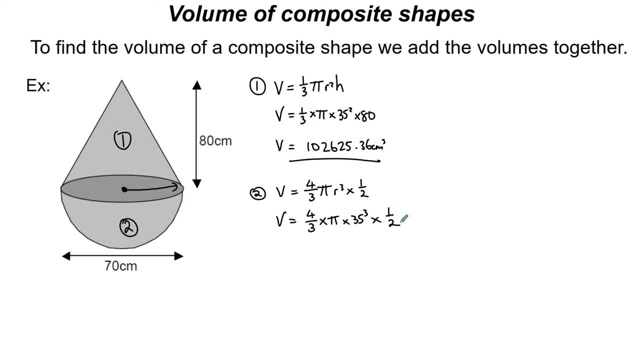 be careful with your powers. times the half, because it's a half sphere. so type in 4 divided by 3 times pi, times 35 cubed, times half 0.5, and we get eight, eighty, nine thousand seven hundred and ninety seven point one, nine and again cm cubed. okay, so for this shape, 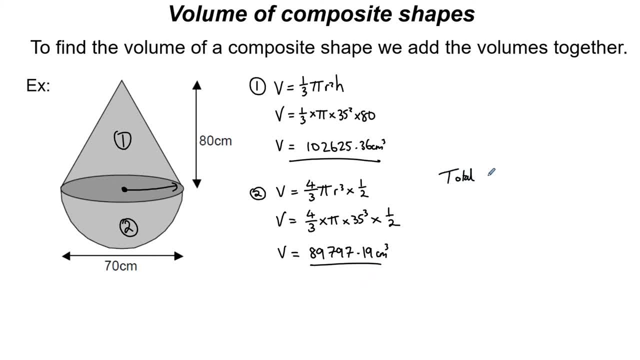 the final step would be to find the total. okay, so the total would just be these two numbers added together. so one oh two, six, two five point three, six plus our previous answer, which i've still got in the calculator. saves me a little bit of typing, so i'm just going to take my answer that: 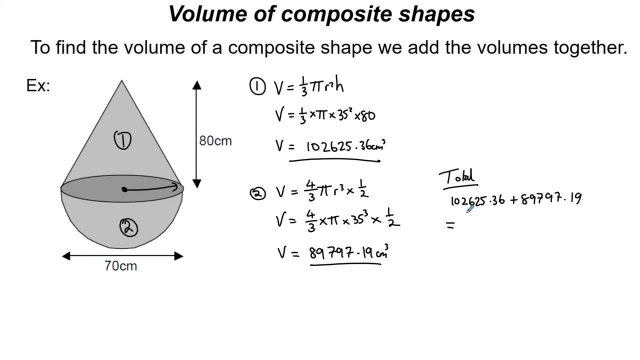 i had one, oh, two, six, two, five point three, six, and add that on to the previous answer, giving me one, nine, two, four, two, two point five, five cubic centimeters. okay, that's all you have to do for constant shapes. if there was three shapes joined together, you would find the volume of each individual shape and add. 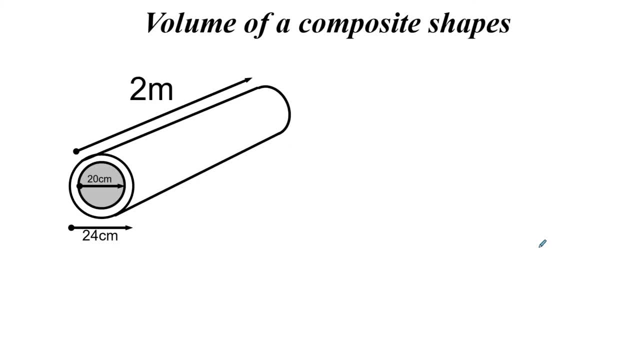 all three together at the end. okay. so what happens if you've got something like this? so what we've got here is a cylinder that's had a nut, a kind of tube shape, so cylinder that has another cylinder cut out from the middle. okay, try to show that as best i can. again, my artwork's not perfect, but 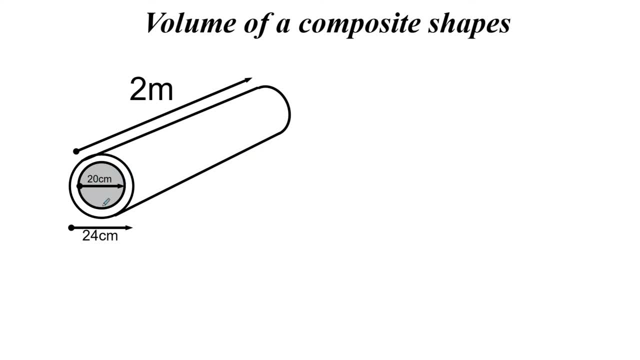 you can see, you've got this kind of outside cylinder that's white, and then inside you've got the kind of tube that's been cut out through the middle, okay, almost like a kind of roll of kitchen roll. and so here we've got again two shapes. we've got the outer cylinder, the bigger, 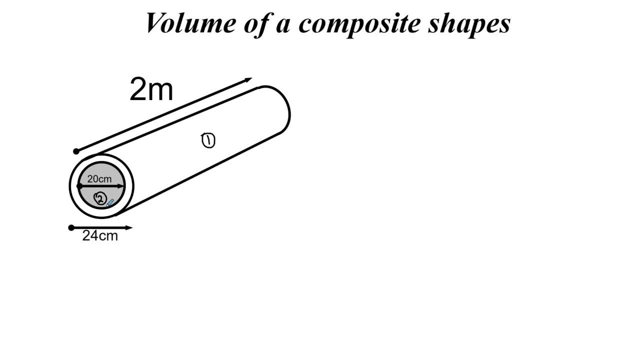 one and we've got the inner one, the smaller cylinder. okay, they are both cylinders. so for shape one we're doing: v equals pi r squared h, so it's pi times now the. we're doing the big one first. so we're looking at this bigger circle on the outside. 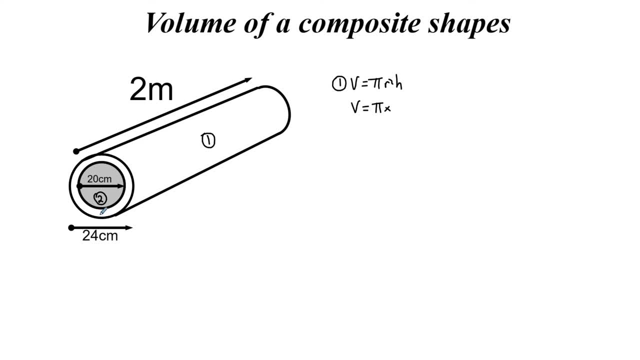 that's the 24 diameter, which means the radius would be from the middle to the outside, which would be 12.. so times 12, squared times the height. now this is how far back the cylinder would be. uh, or how far it would stand if it was standing up. now, watch out for this. units have got to be. 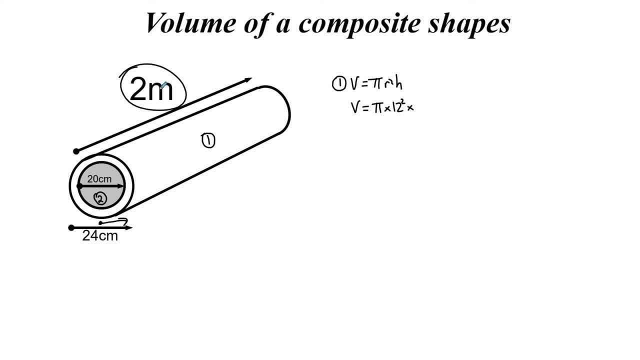 consistent, okay, and most of these are centimeters. we can't use a mixture of centimeters and meters or it'll give us an inconsistent answer, okay, so so two meters is 200 centimeters, 100 centimeters in every meter. so times 200 at the end here. 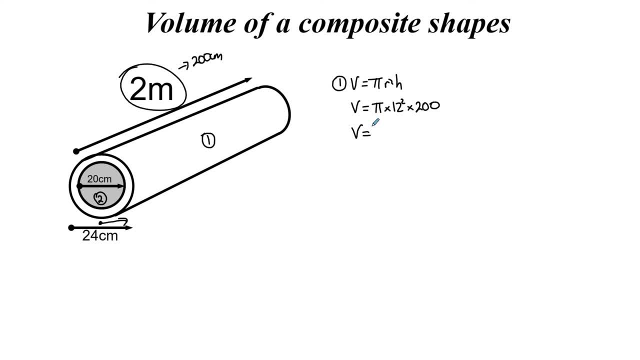 okay. so it's pi times 12 squared times 200. the first part, that's 90, 477, 0.87. again, we're just sticking with two decimal places just now. shape two is that again a cylinder. so v equals pi r squared h, so it's pi times. now we're looking at the smaller circle here for the. 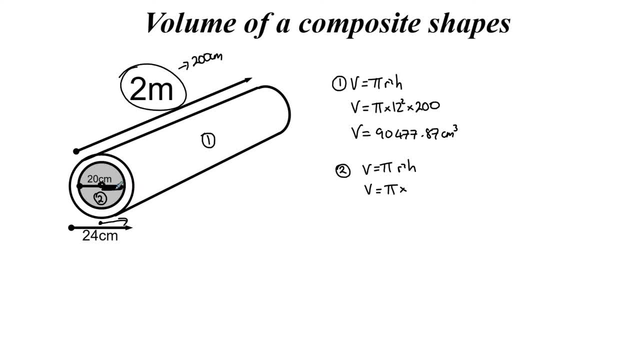 inside cylinder. so the radius of that would only be from there to there, which is 10 squared, but the height, or how far back the circle goes, is going to be 200 step. so v equals pi times 10, squared again, to type into your calculator, times 200, and that gives you 62 000.. 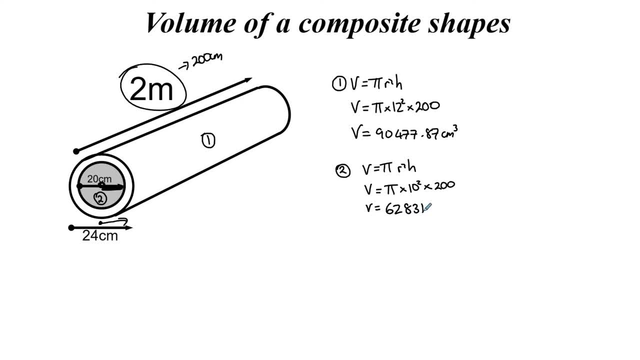 so we've got here. the total volume is going to be 831.8, 5 cm cubed. okay, and this time, because you've got a shape cut out of another shape, when you want to find the kind of resultant volume you're going to actually take away. okay, so the volume of that kind, 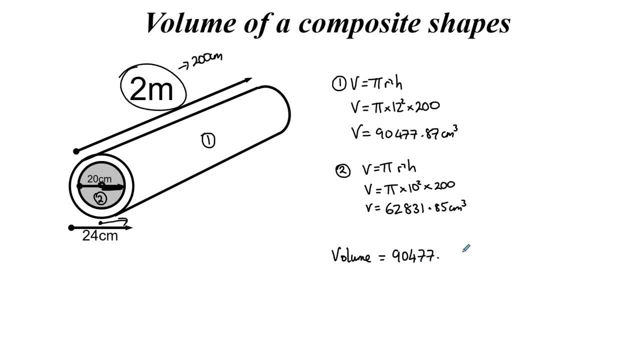 of white tube shape, there is going to be the bigger one. ninety thousand four hundred and seventy seven point eight seven. take away the smaller one. okay, so we're going to do 90,477.87 minus the previous answer. that's going to give us 27,646.02 cm- cubed or cubic centimeters. okay, and that's our resultant volume for. 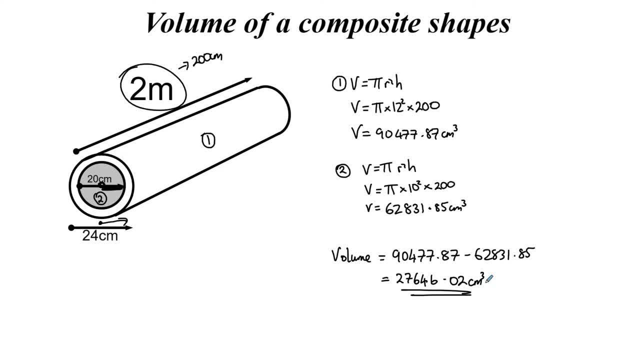 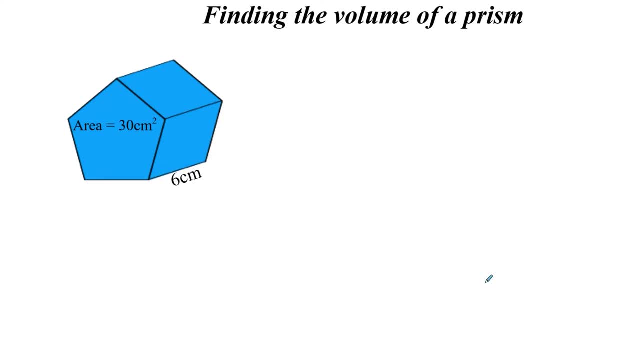 the white part of that shape. okay, so next i'm going to look at is finding the volume of the prism, and quite an easy process as long as you are kind of aware of how prisms work. now we've actually already looked at a few prisms with the cuboids and the cylinder, so a prism is a shape. 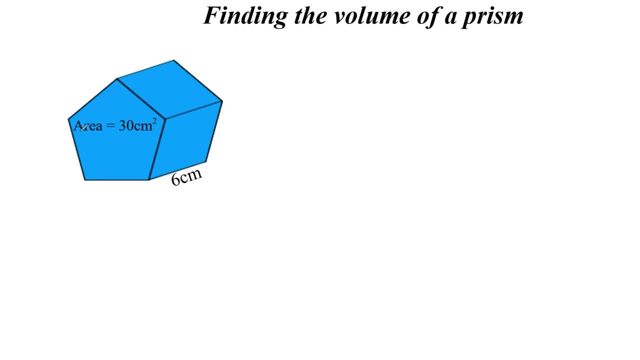 that has the same kind of cross section. so this kind of front face is a pentagon, a regular pentagon, repeating all the way throughout. it doesn't, the shape doesn't get smaller, it doesn't taper in and it doesn't get wider and it just stays the same kind of size all throughout. so 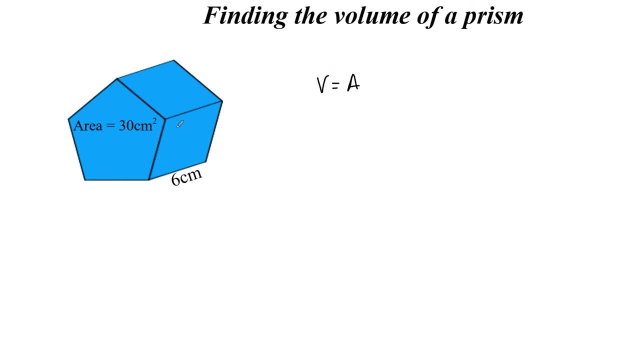 the volume of any prism is the area of the cross section. so the area of this front face times the length of the shape, how far back that cross section goes. so volume here would be 30 times 6. nice and easy, which is 180 cm cubed. okay, you notice that the gate. we already had the area. 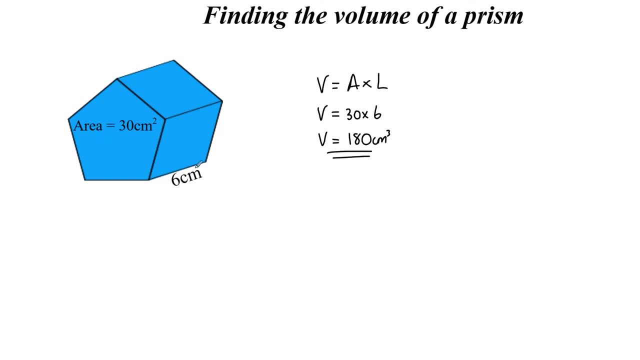 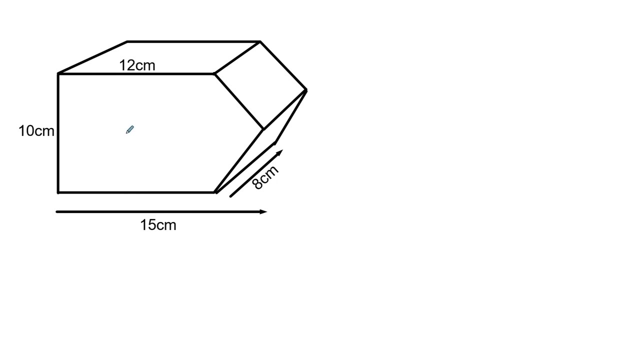 of the front section, so it's just the area of that times the length of the shape. okay, so nice, easy formula. prisms are nice and straightforward. however, you're not always going to be given the area. so if you look at something like this, which is going to be our final shape today, this is a prism. 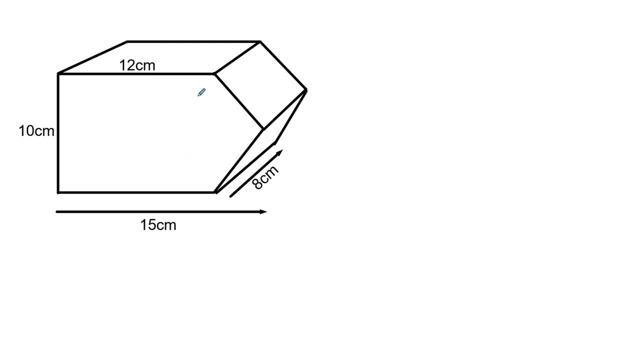 you've kind of almost got this house on its side or arrow kind of shape here. it's not a shape we recognize. okay, i don't recognize this front shape. we're not told the area of the front section, so we don't know what this is. instead, what we're going to look to do is we're going to look to. 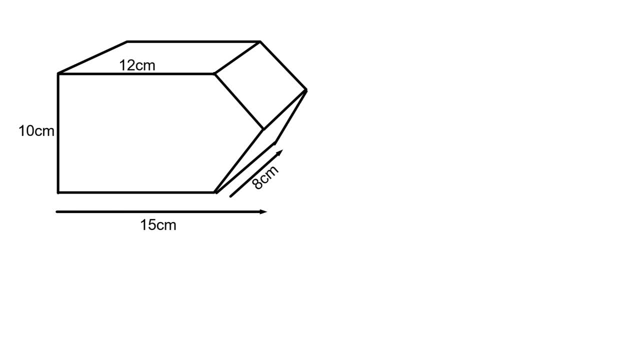 split it up into shapes that we do recognize. okay, they are going to be prisms, because the shape stays the same kind of, it's the same cross section all the way through. but what we're going to do is, if we split it down here like that, then you can now hopefully see that that. 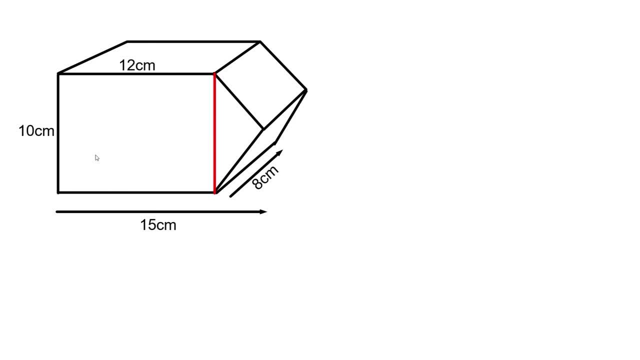 is a cuboid or a rectangular prism and a triangular prism here, okay, and from that we can just use what we know about prisms to find the volume of each shape individually. so we'll do one and two, just like we did with the composite shapes, and then add them together. so 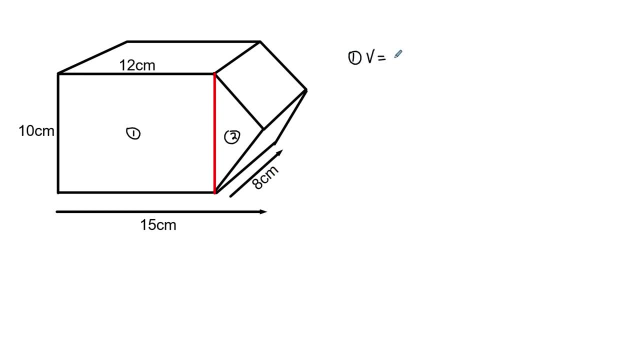 shape one is a cuboid, so it's length times the breadth times the height, lbh. so it's length, sorry, length of the cuboid. so here if we look at the cuboid, we're just focused on this section. here the length of the cuboid would be 12. be careful you don't pick the 15. the 15 is for the whole shape. 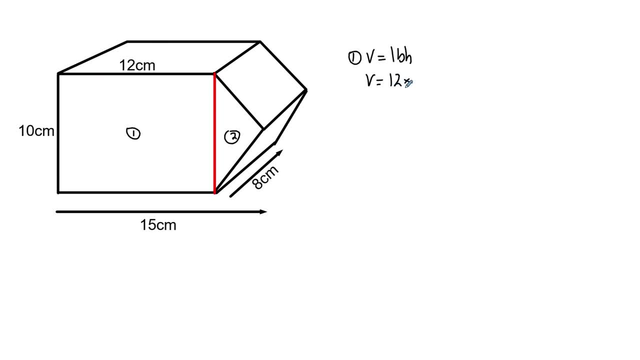 okay, the length of the cuboid part is 12.. so it's 12 times the breadth of the cuboid, which is 10 times how far back it goes at the height of the cuboids. eight, okay, and we're taking that from this section down here. so that part would be eight. so twelve times ten times eight. 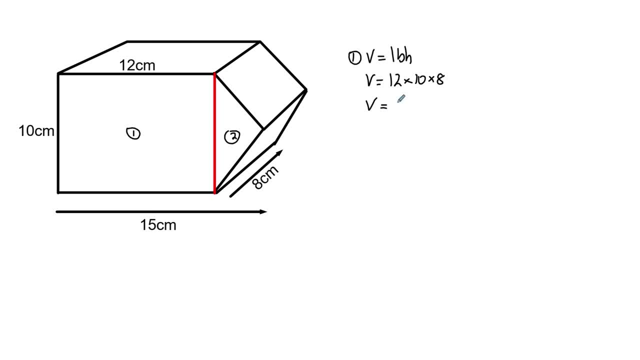 so that should give you 960.. cm cubed for that cuboid section. okay, that's the first part. the triangular prism: now we've not covered this explicitly yet, but we know that the area of a triangle is a half times the length times the breadth, so the volume would be a half times the length times the breadth times the height. 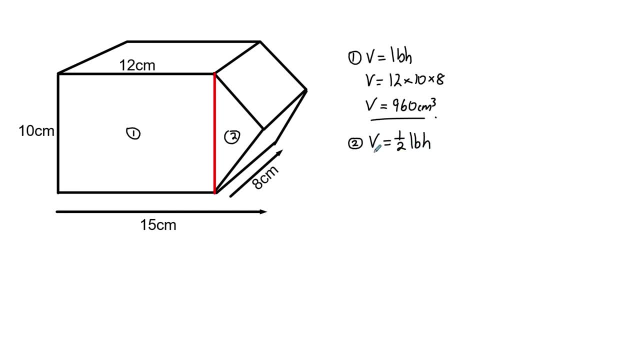 again, it's very similar to the relationship between area of a rectangle and area of a triangle. so if the area of a rectangle is a half times the length times the breadth times the height, the volume here of the cuboid was lbh. the volume of a triangle is a half lbh, so it's a half times. 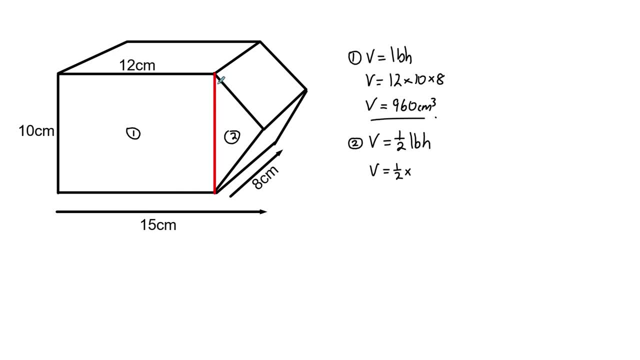 so the length again, just as long as you pick the correct dimensions, this is what you have to focus on. so i'd say length. here i'm going to tilt my head and look at this as being the length of the triangle, which is the 10, the breadth. i'm going to call this distance here now, here, from here to here. 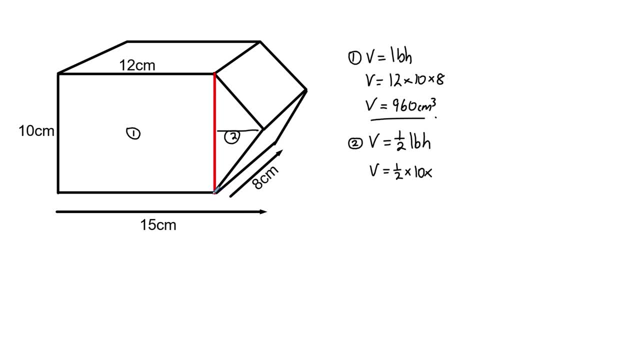 it's not 15, it's that distance between that part and the end. okay, so this part was 12, this part is 15. we're looking for the difference. so 12 add 3 gives us 15. so it's 3 or 15. take away 12. 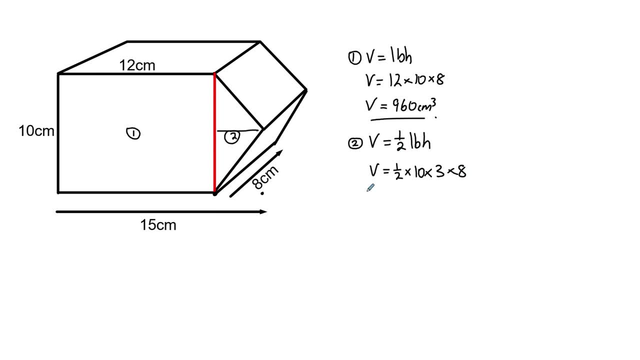 and the height of the shape is still the same. it's been pushed a depth of 8 centimeters. so v equals half times 10 times 3 times 8, and that would give us: half of 10 is 5. 5 times 3 is 15.